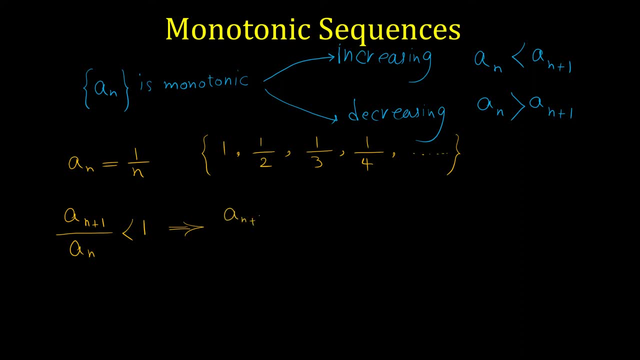 so we have to make this ratio and we have to show that this ratio is less than one. a sub n plus 1 is 1 over n plus 1 and a sub n is 1 over n. if we simplify this, we have 1 over n plus 1 times by reciprocal of denominator, which is n. 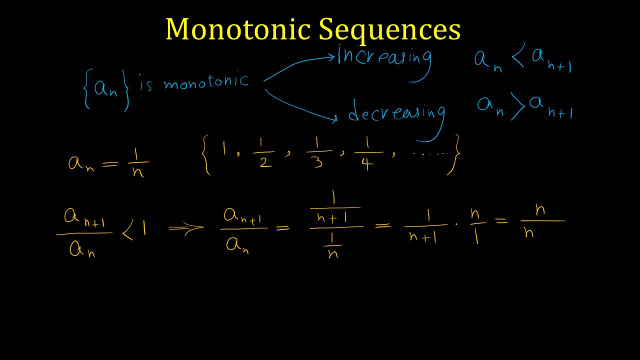 over 1, which we can multiply top by top, bottom by bottom, and we get to n over n plus 1. this fraction is less than 1 because the numerator of this fraction is less than the denominator, so this ratio is less than 1, and so this sequence is a decreasing sequence. 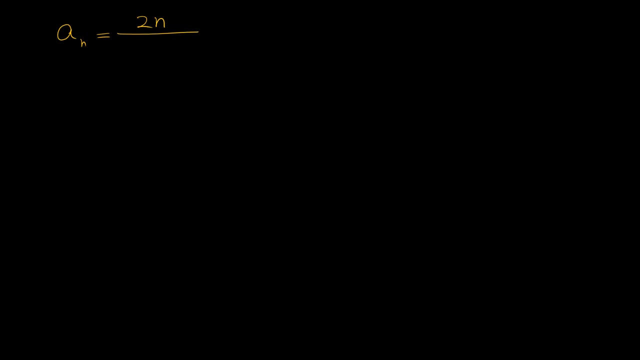 now consider this example: 2n over 2n plus 1. the first term of this sequence is 2 over 3, the second term is 4 over 5, the third term is 6 over 7, the fourth term is 8 over 9, and so on. 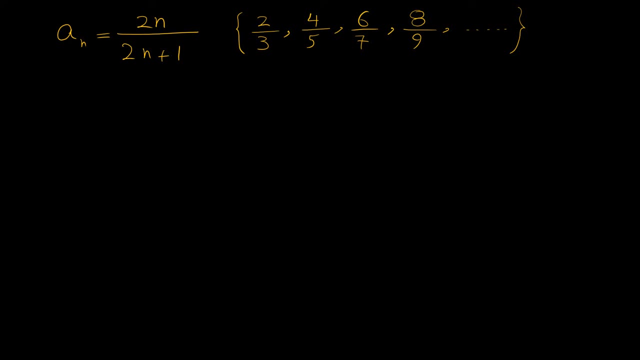 while looking at the terms of this sequence, we can guess that this sequence is an increasing sequence. but to prove that this sequence is increasing, we have to show that a sub n plus 1 over a n is greater than 1. first let's make this ratio: a sub n plus 1 over a n is greater than 1. 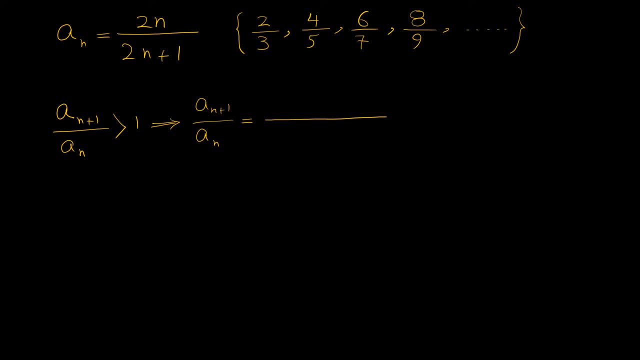 now imagine to calculate the constant of a n over n of a caseized function. the f x sub 1 sub n, 2x over 2 n plus 1 can be obtained by substituting n plus 1 in the n-term formula. if we substitute n with n plus 1, we get 2n plus 1 over two times n plus plus 1 over 2 times n plus 1 plus 1 over two and over 2n plus 1. if we multiply two, in the end we get igual to n 3x1 over n unlocked. and then we get one n squared over 2n plus 1 minus one n plus 1 over the n plus when we substitute n and we get two functions here, we get two xn plus 1.